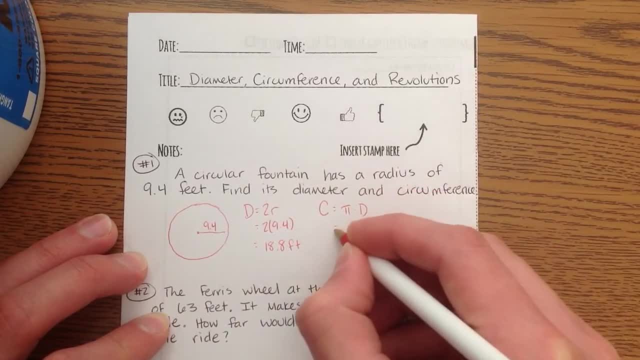 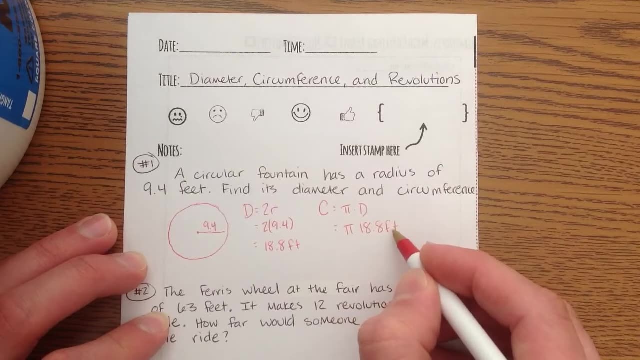 Circumference equals pi times the diameter. so we get pi times 18.8 feet. Now, if you want an approximate answer, you could do 18.8 times 3.14, but we'll just keep it as 18.8 times pi feet. Okay, so the circumference equals that and the diameter equals that. 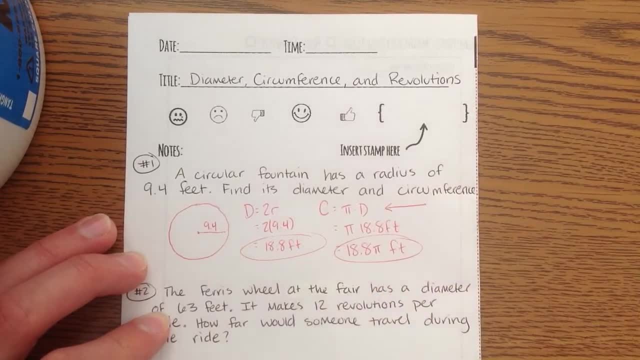 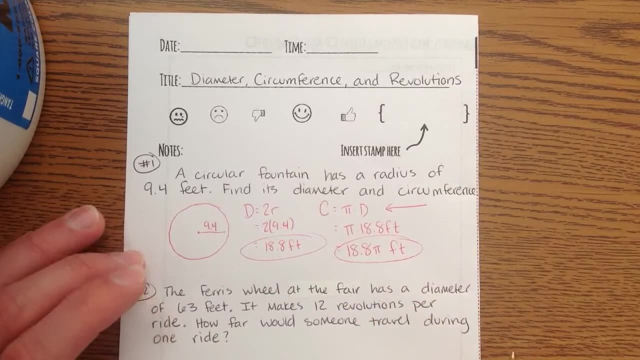 and the key was just to remember from today's activity And yesterday with the coffee filters, that circumference equals pi times diameter. Okay, multiply that if you like, but we'll keep it there. Two: the Ferris wheel at the fair. 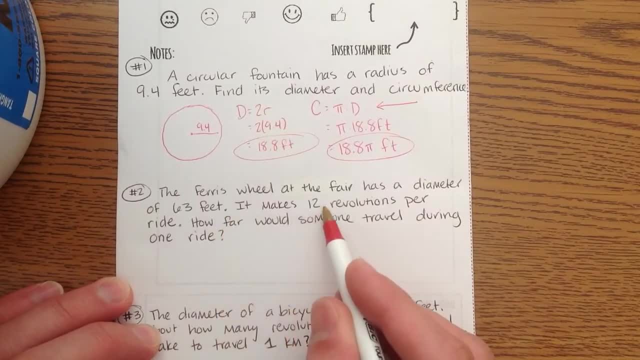 has a diameter of 63 feet. It makes 12 revolutions per ride. How far would someone travel during one ride? Well, so a revolution is just one full time around. okay, It's one complete turnaround. So I'm going to draw this Ferris wheel. I'm going to draw this Ferris wheel. 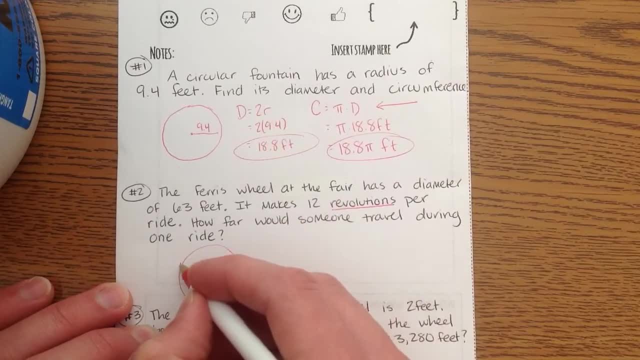 real quick. okay, Here's my Ferris wheel. These are going to be the little people who ride along the edge of it, right? So these are little capsules that go along the edge, okay, And maybe my Ferris wheel has, like some, stands here like this. okay, So that's my. 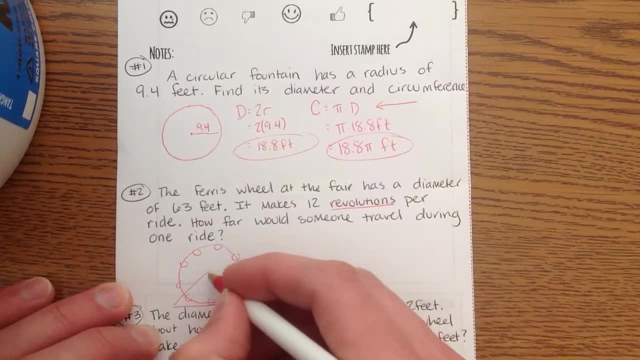 Ferris wheel. all right, You could probably draw a better one. Draw a better one than me, because you guys are better artists than me. So this is the Ferris wheel and it has a diameter. okay, Of what? 63 feet. 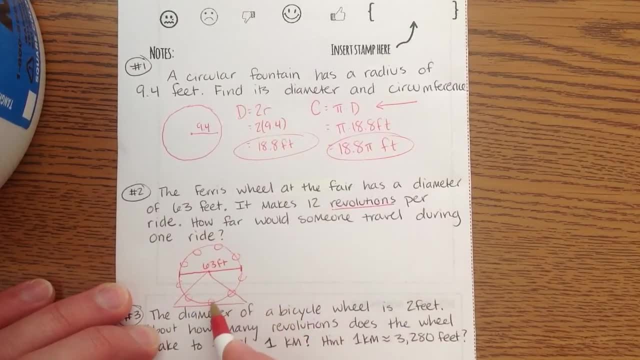 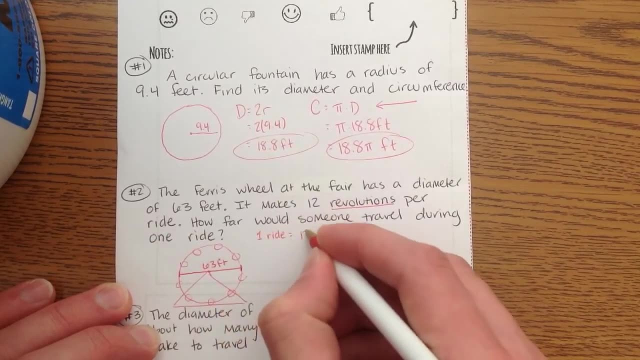 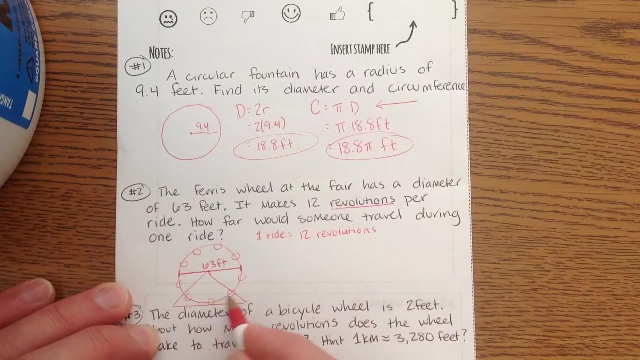 63 feet. So what do we need to know? We need to know how far they travel around on one ride. okay, But one ride equals 12 revolutions. Now here's a key: Whenever you talk about revolutions, that's a complete turn, and a complete turn around the whole thing would. 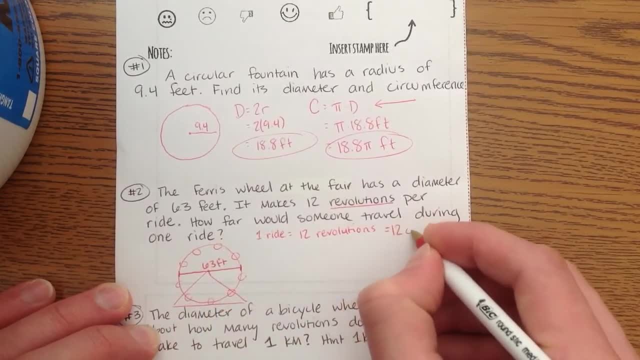 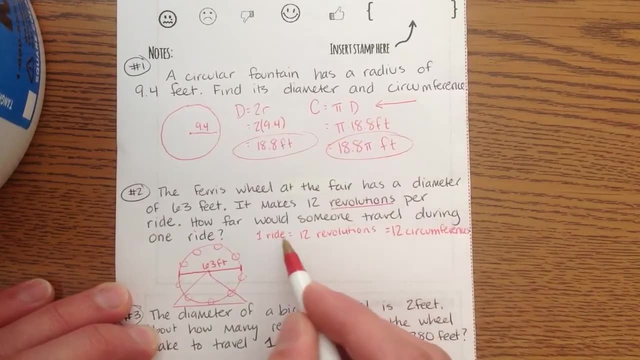 be a circumference, So that equals 12 circumferences. right, And that's really the key that you need to take away from this. And it goes around one time. It goes around the circumference once. Well, let's find the circumference real quick. The circumference equals pi times the diameter, which equals 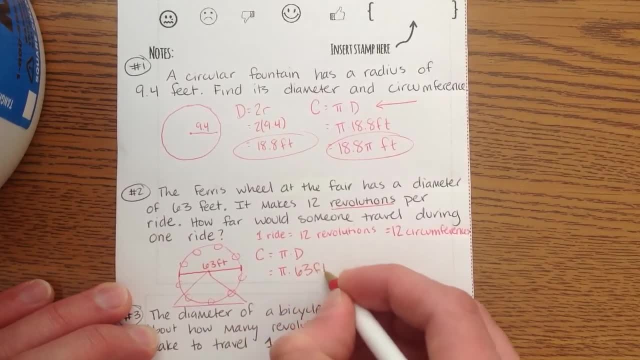 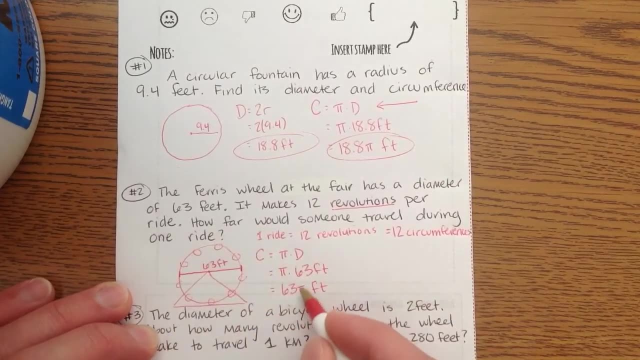 pi times 63 feet, okay, And we're just going to keep it as 63 pi feet. So that's how long, and we could multiply by 3.14 to get an approximate value of one circumference all the way around. 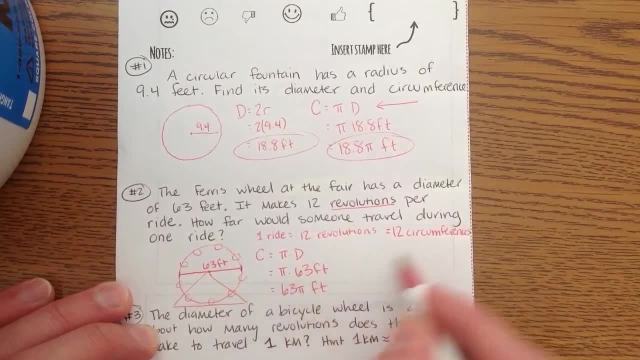 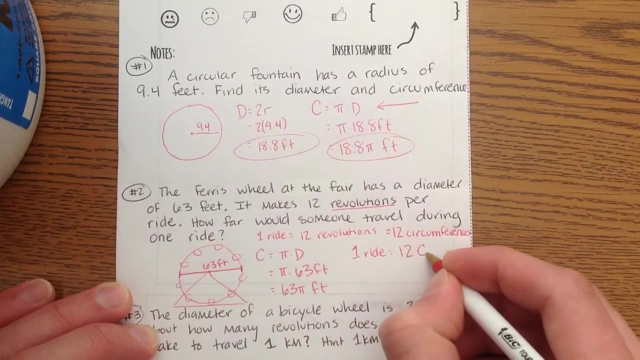 And how many times do they go around? Well, they go around 12 times, because the ride lasts 12 revolutions, 12 times around the Ferris wheel. So the full ride, one ride- equals 12 times the circumference. Well, what is the circumference? It's this which is. 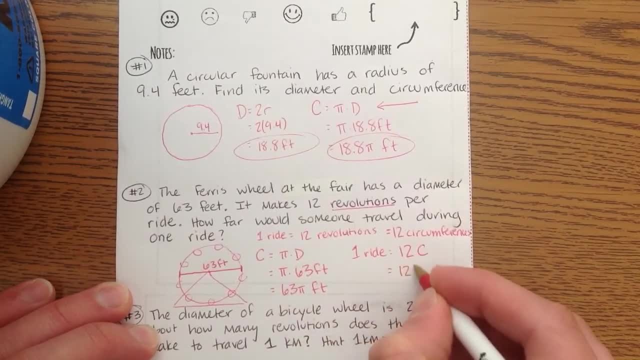 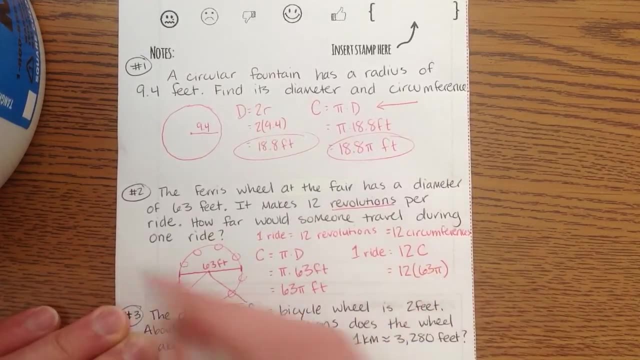 63 times pi. So one ride equals 12 times 63 pi. okay, So we have to multiply 12 times 63.. I'll do that over here, because I have some space over here. 63 times 12, and we 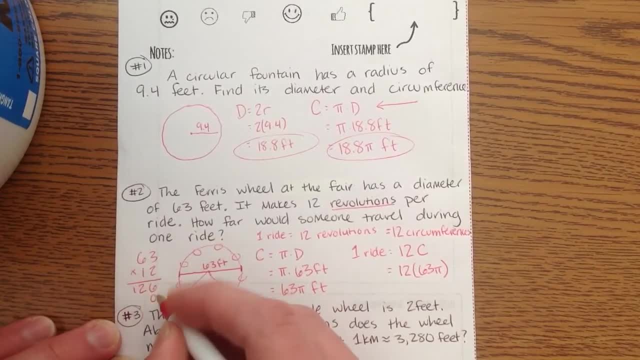 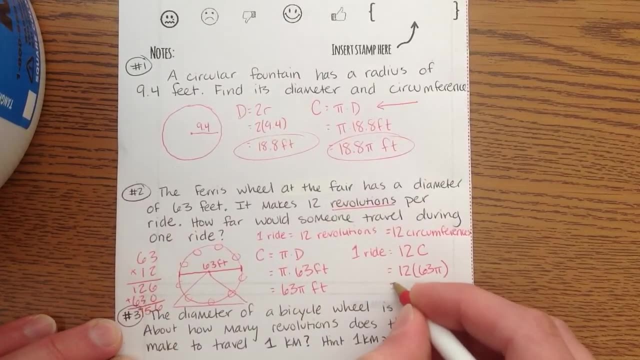 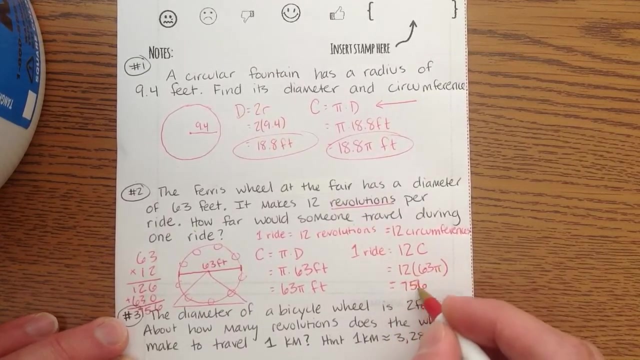 have 6,, 126,, 0, and 63.. We're going to add that up: 6,, 5,, 7,, 756.. So this equals 756.. Are we done? You can't leave this off. We haven't multiplied pi yet, So we have to. 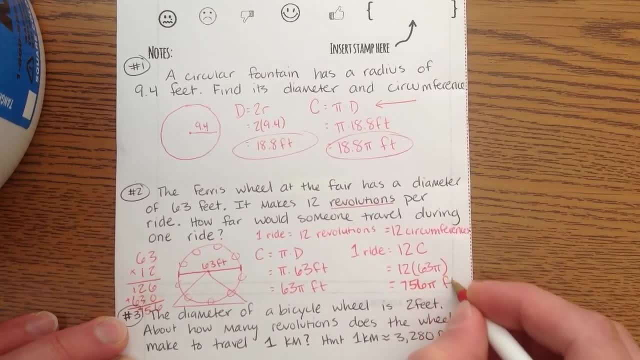 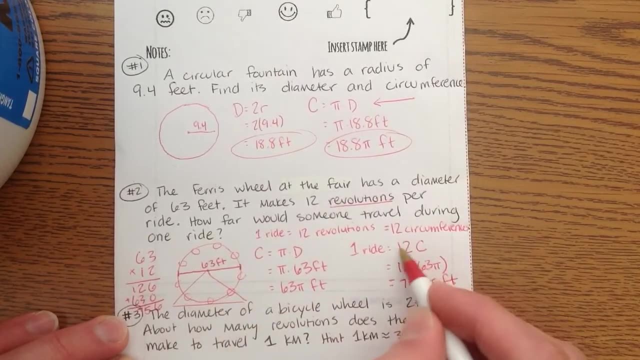 do 756 times pi feet. okay, And that's the full distance. they would go on one turn. No, on 12, 12 circumferences. So when it says revolution they would go on one turn, and when it says revolutions you have to multiply by the circumference the amount of revolutions. 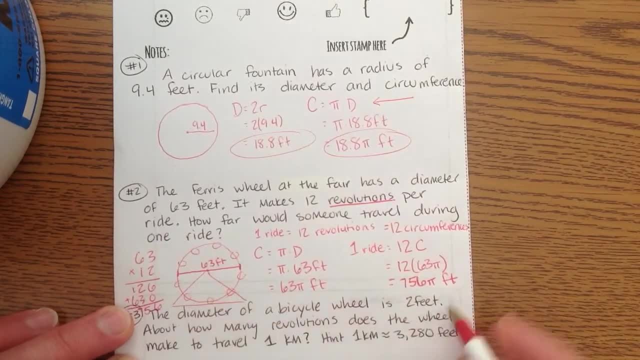 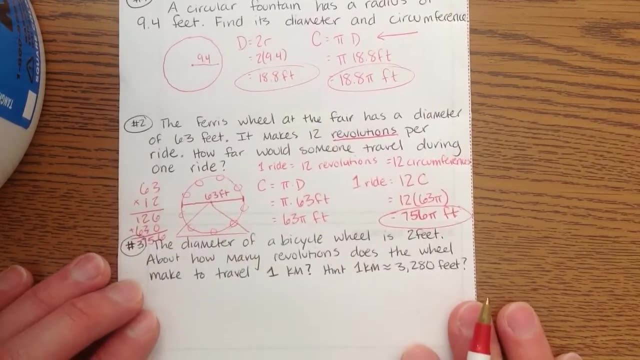 because that's the amount of times it goes around, That's the amount of distance they would travel. So we get 756 times pi feet, and again you can multiply by 3.14.. Let's do one more, This one. think about what we just did, okay, And think about this new problem. 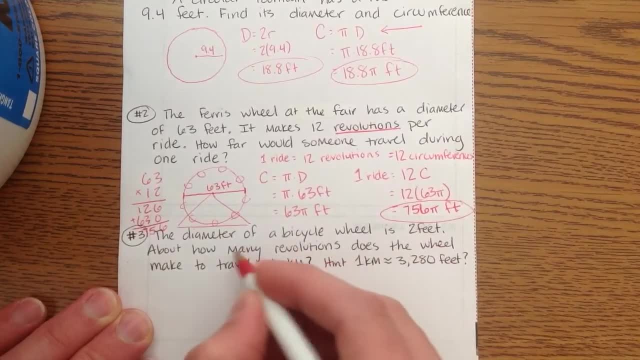 The diameter of a bicycle wheel is 2 feet. About how many revolutions? That's the question. How many full turns does the wheel make to travel 1 kilometer? Hint. 1 kilometer is about equal to. this means approximately equal, because it's a squiggle equal sign, so approximately. 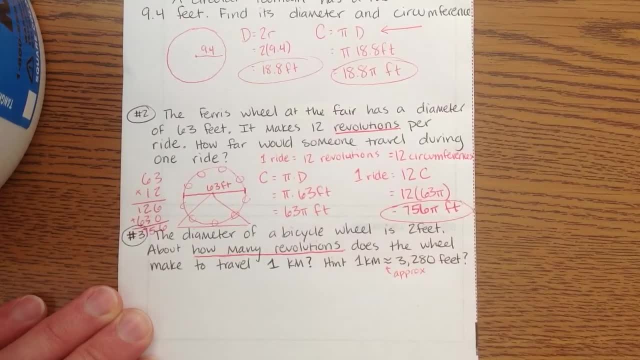 equal to 3,280 feet, okay. Well, let's do it real quick. Let's draw a bicycle wheel. So here we go Again. you could probably draw a better one than me, but we'll have some spokes here like this: on my bicycle wheel. That's my bicycle wheel, okay, And the diameter? 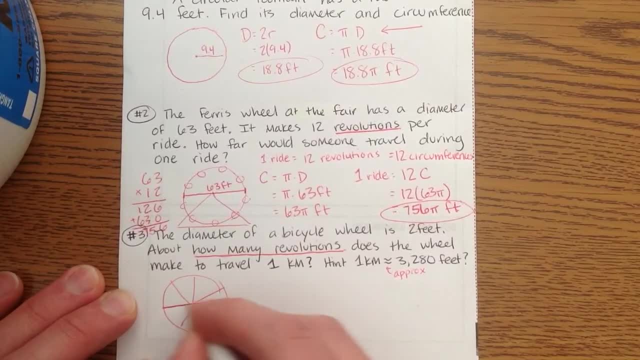 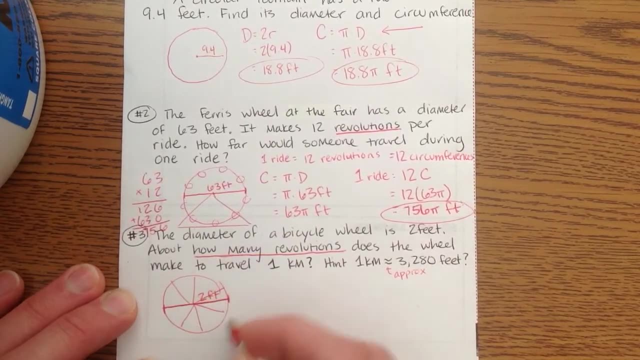 of this thing. so from one side straight to the other. this will be my diameter. okay is 2 feet. 2 feet On one turn with the bicycle wheel goes around one time. how far does it go around? It goes.